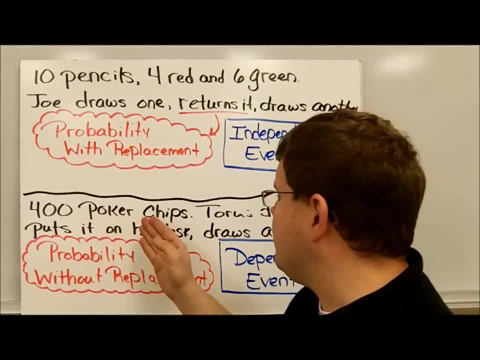 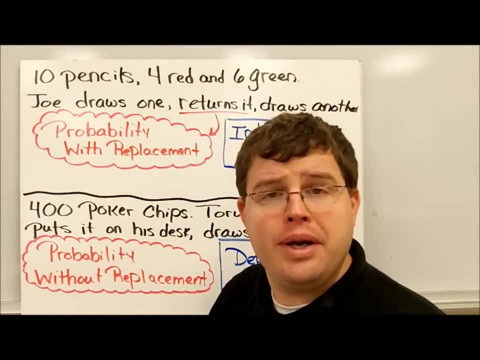 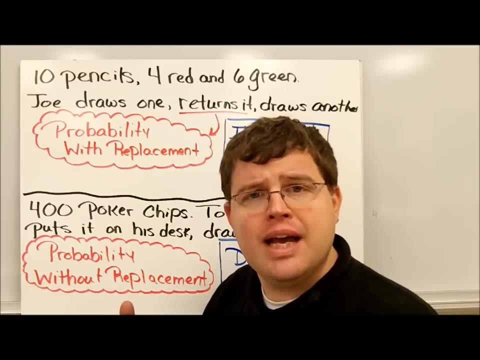 the second time. On the other hand, here we have 400 poker chips and Taurus draws out a poker chip and puts it off to the side. Well, now there's only 399 poker chips left in that box And because we didn't put it back, what happened the first time had a big impact on what could. 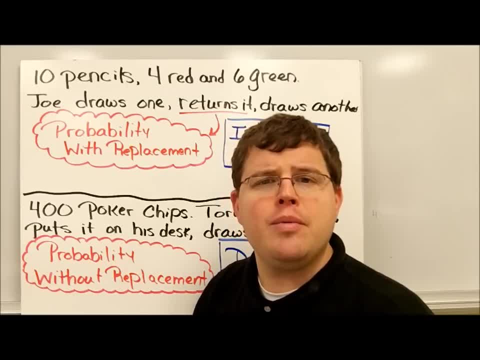 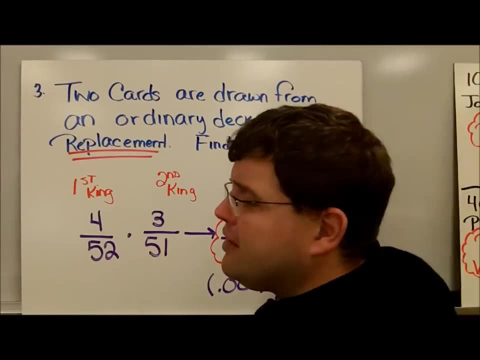 happen the second time. As a result, we have probability without replacement. Since we didn't replace it, the first event impacted what could happen the second time. We have dependent Debts of the Daarимся. Take a look at this example. This is example number 3.. We have two cards. We're drawing. 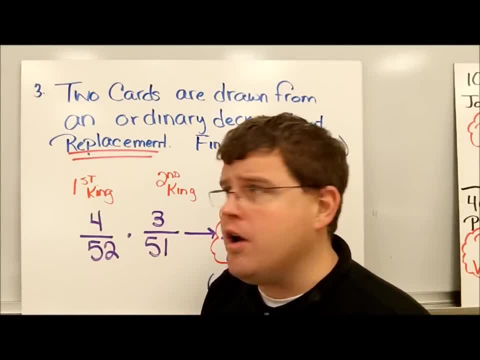 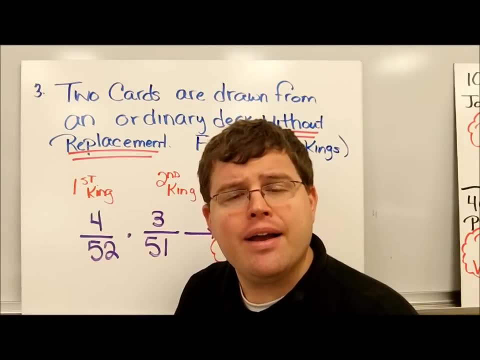 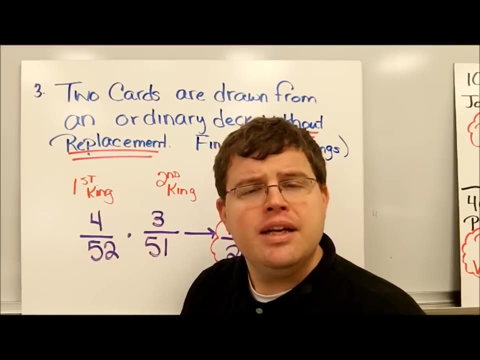 cards out of a deck And we want the probability of drawing two kings. Now we're going to draw the first card out, but we're not going to put it back. That's probability without replacement, Because I didn't put the first card back. things have changed and therefore 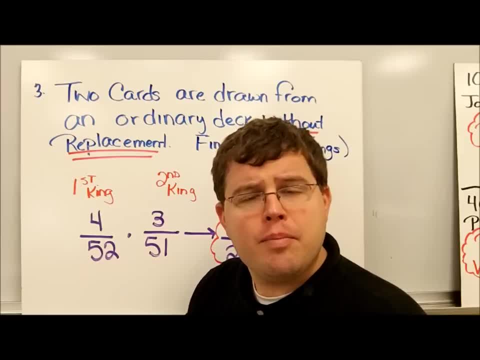 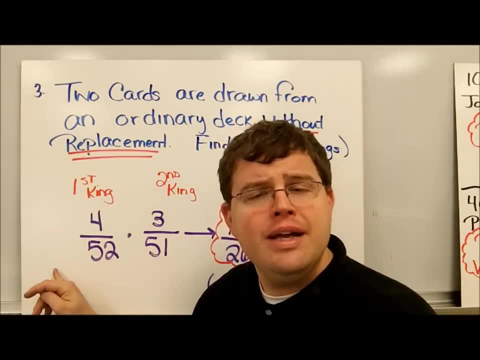 we have dependent events. The probabilities are going to change a bit. The probability of getting a king: the first time there were 4 kings out of 52 cards, So 4 out of 52 is the probability of the first king. Now, if I drew that king, there's now only 3 left. 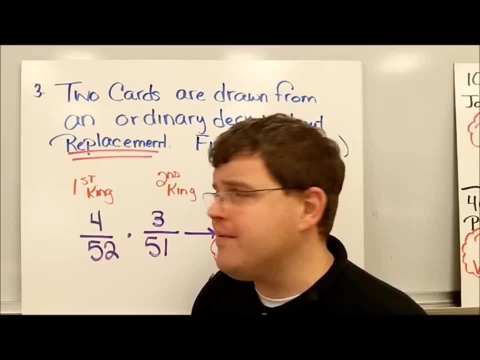 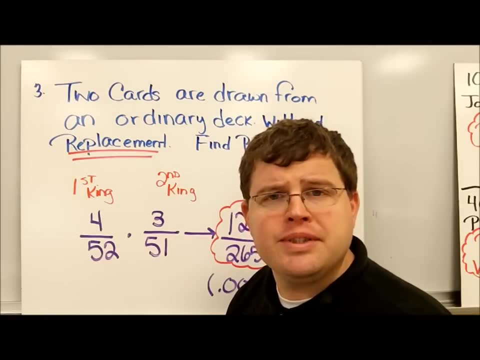 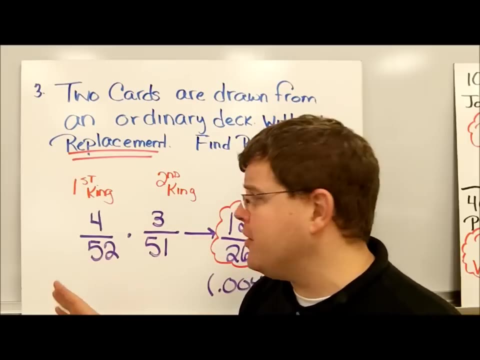 in the deck and there's only a total of 51 cards left, And so the probability of getting a king the second time is 3 out of 51.. We know the counting principle says that if we get a king and a king the word and tells us to multiply, we multiply the probabilities. 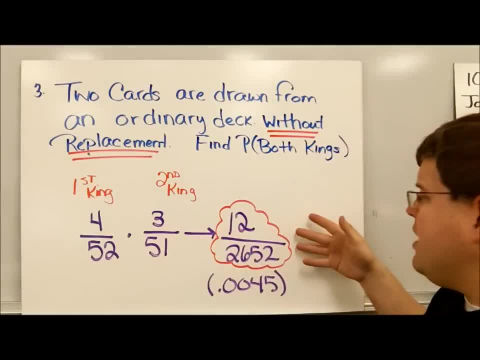 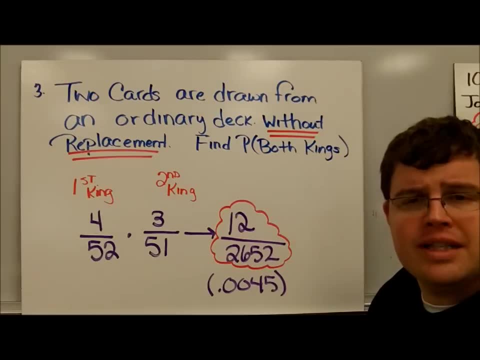 4 over 52,, 3 over 51, and we get 12 out of 2,652, or roughly a half of a percent. So it's not very likely that you're going to get a king and then another king. It could. 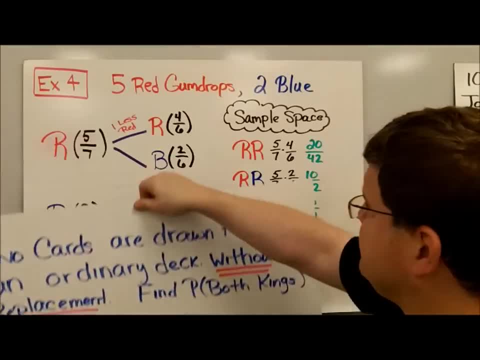 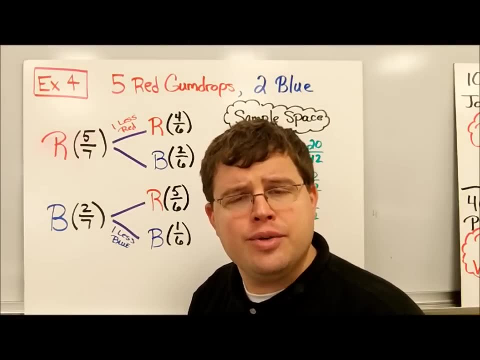 happen, though. Now it's very helpful, when you're dealing with probabilities that are probability without replacement, to create a tree diagram. A tree diagram really puts everything in order, helps you stay very organized. Take a look, here We have a bag of gumdrops. 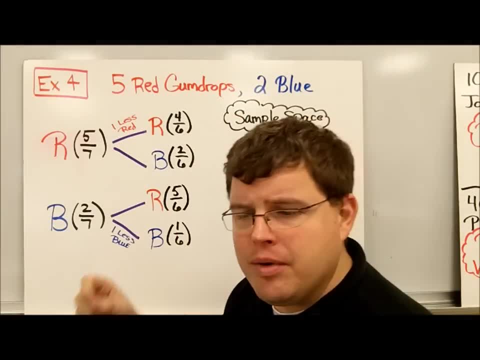 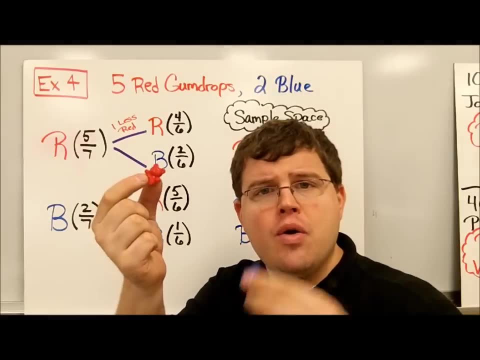 We have 5 red ones, 2 blue ones, And we're going to reach into that bag and we're going to pull out a gumdrop And one of two things could happen: I could pull out a red one or I could pull out a blue one. Probability of a red was 5 out of 7.. Probability of a 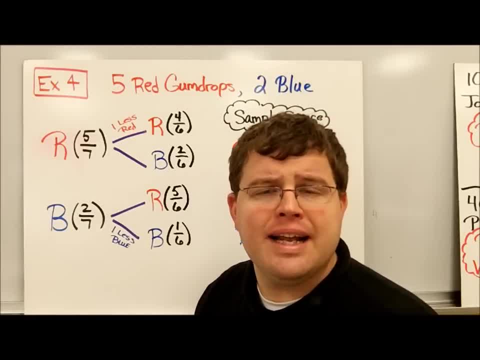 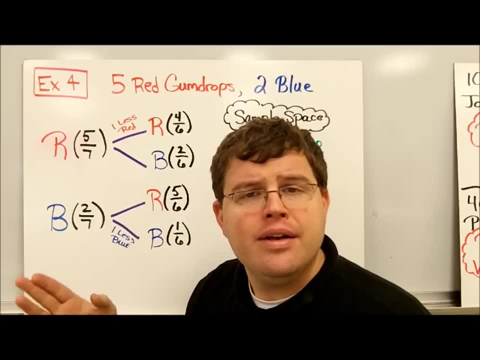 blue was 2 out of 7.. Now here's where things get a little trickier. Let's suppose I drew the red one out first and then I ate it. I didn't put it back. Well, what's left in the bag? Well, there are now. 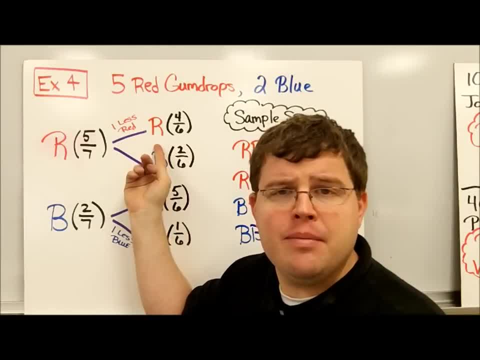 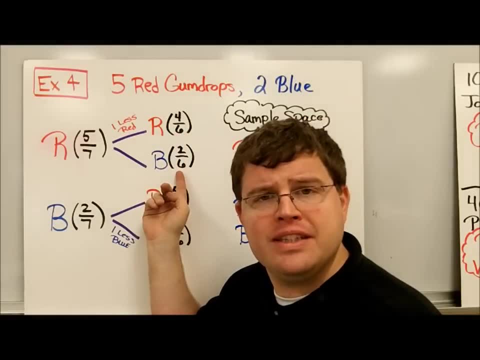 4 out of 6 red ones left in the bag. Notice, there's only 6 left because I ate one and there's only 4 red ones, And there are now 2 out of the 6 that are blue On the other. 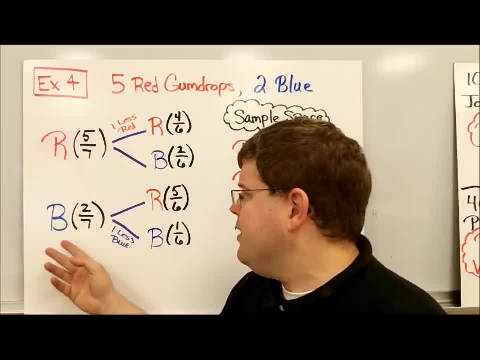 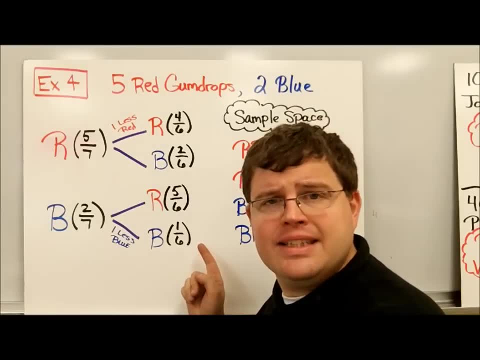 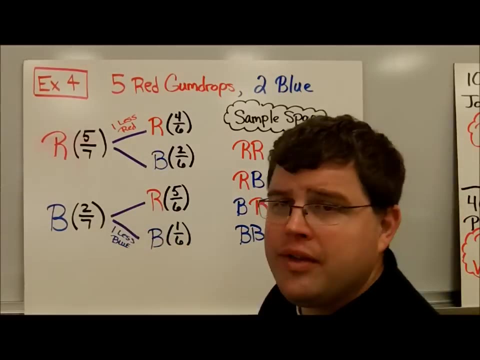 hand if I ate the blue one. I drew the blue, I ate it. There are now only 6 gumdrops left in the bag. 5 of the 6 are red, 1 of the 6 is blue, And so you can see how the probabilities changed from here to here and all the way through. 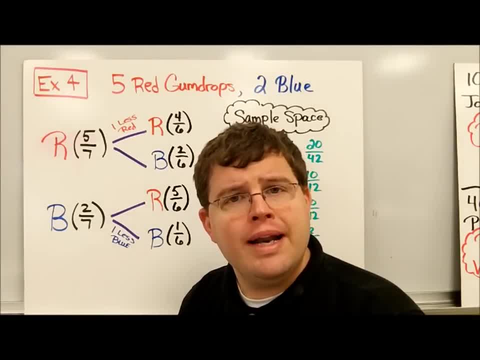 because they were dependent events. If I drew a blue one and ate it, I couldn't well draw that blue one again. Now we'll use the counting principle to write our sample space. We could have gotten a red one and a red one. That's a red one, That's a blue one, That's a blue one, That's a blue. 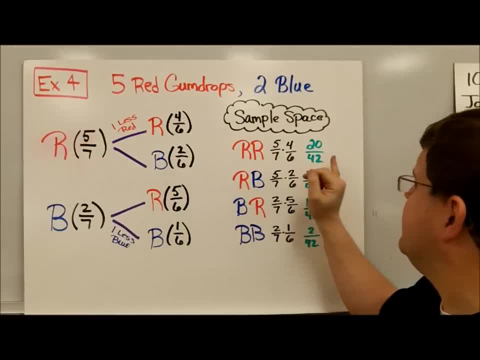 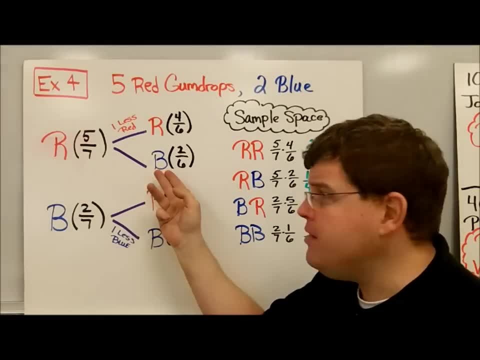 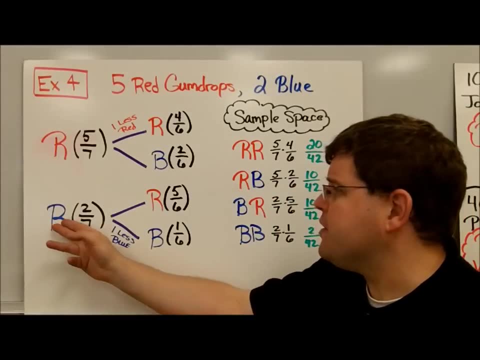 done a red one and then a blue one. 5 out of 7.. 2 out of 6 multiplied together, That gives me 10 out of 42.. I do the same for the blue and the red And the blue and the blue. 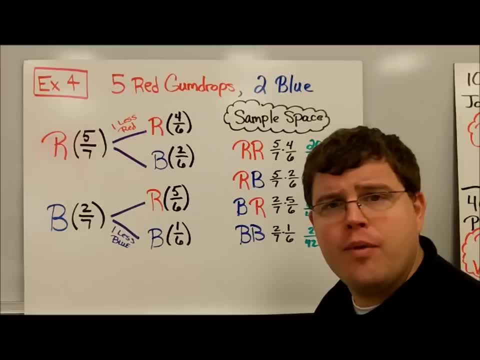 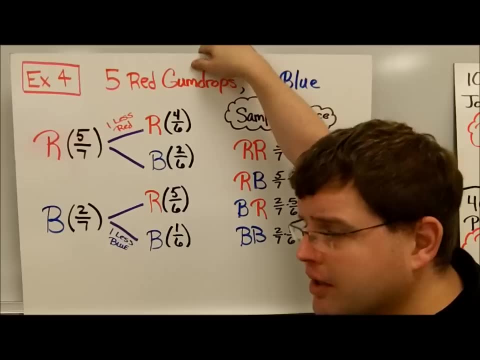 I get probabilities of 10 out of 42. And 2 out of 42. And I use that information to answer the questions that they want me to answer. Let's take a look at some of those questions. The first thing they ask me is: what's the probability that both gumdrops were red? 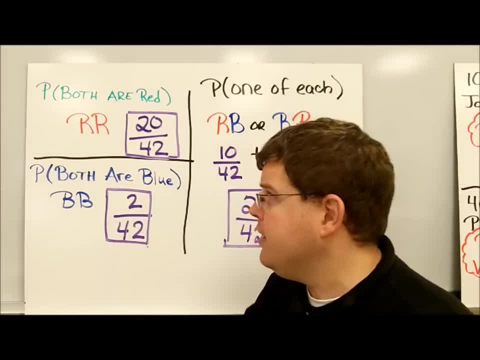 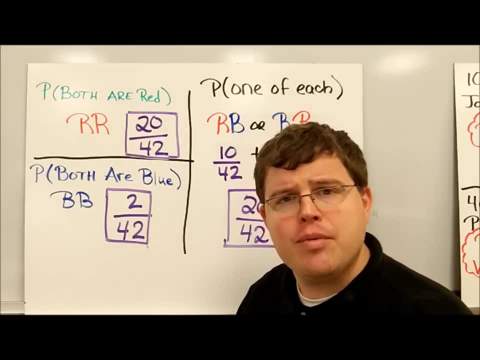 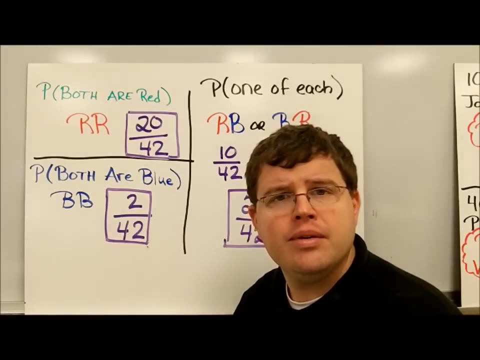 Well, that happened in my sample space when I had RR. The probability was 20 out of 42.. What's the probability that both are blue? That happened when I had BB And the probability of that, according to my sample space, was 2 out of 42.. 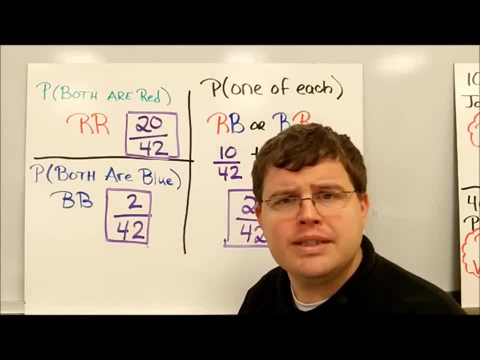 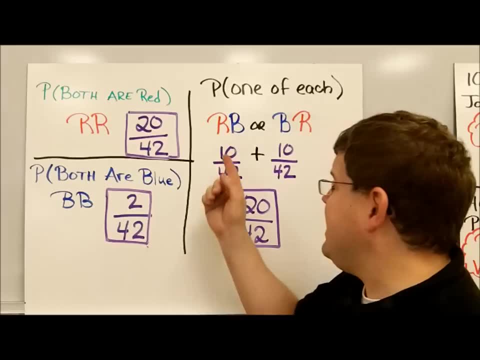 Now we've got to think a little bit here, because on the third one they ask us what's the probability that we had one red and one blue. Well, that happened in two different places. It happened when we got the red one, then the blue one. 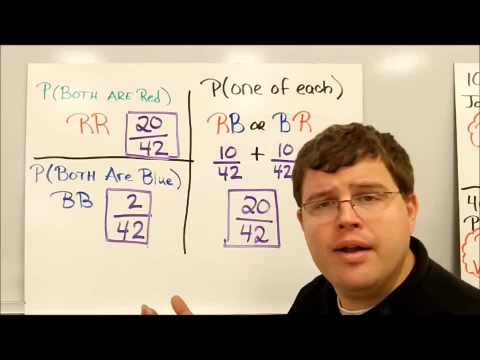 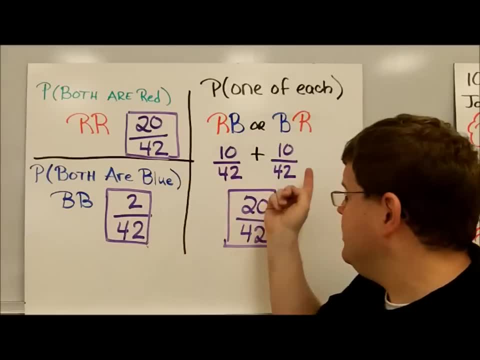 It also happened when we got the blue one and then the red one, And so we have to add those probabilities together: 10 out of 42 times for red then blue. 10 out of 42 times for blue then red, that's 20 out. 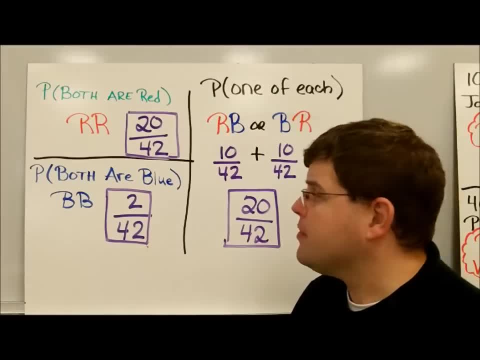 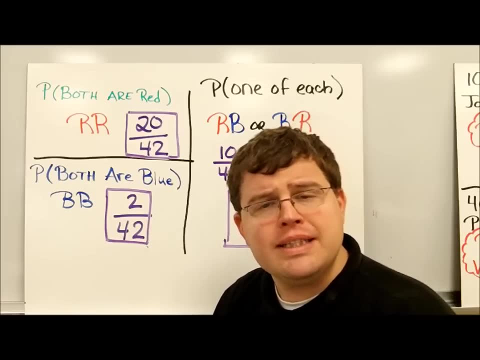 of 42. That gave us a red and a blue. That's the basics of probability without replacement. There's several examples that come up next in the notes packet and let's take a look at those. I'd like for you to try those and then compare your answers to those that I'm going to put. 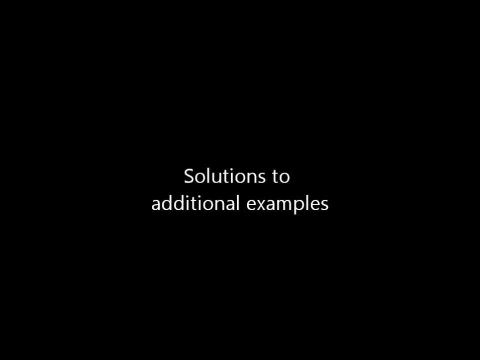 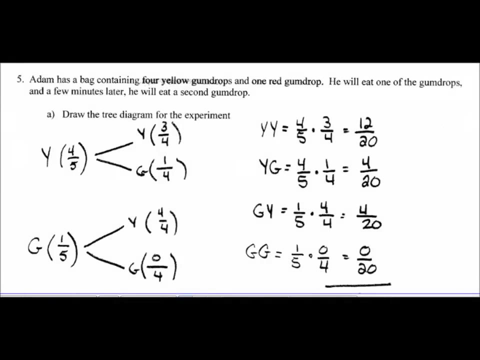 on the screen in just a moment. Example 5 is another example involving gumdrops. We have a bag that has five gumdrops in it- four yellow and one red. It says that Adam will draw a gumdrop, eat it and then, a few minutes later, draw a second. 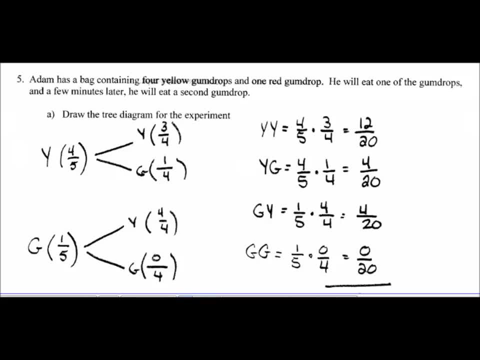 one Because he didn't replace it. we have probability without replacement. We have dependent events. The tree diagram shows the probabilities associated with all the possibilities: A yellow and then a yellow, a yellow and then a green, a green and then a yellow or a green. 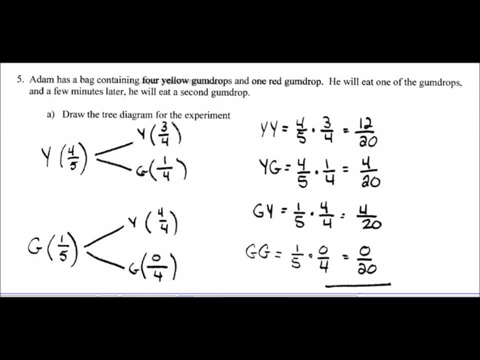 and then a yellow, Another green. Notice. the most interesting thing here is down at the bottom, where we have green green Because there was only one green. it's impossible for Adam to reach in and eat two green gumdrops from this bag. 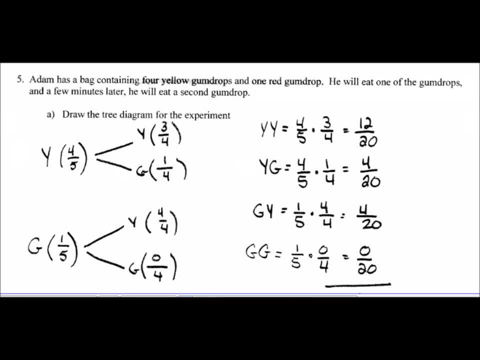 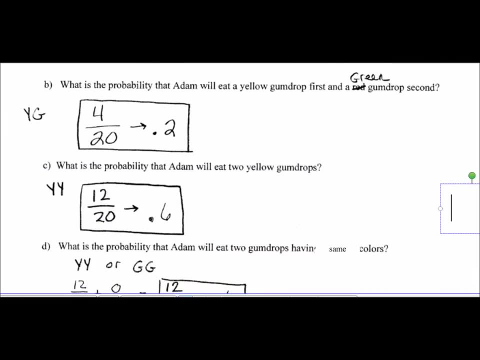 Now let's use these probabilities that we've listed over in our sample space to answer some questions. First question is: what is the probability that Adam will eat a yellow gumdrop in a green gumdrop? second: Well, That happens when we have the events Y, G, Yellow, green. 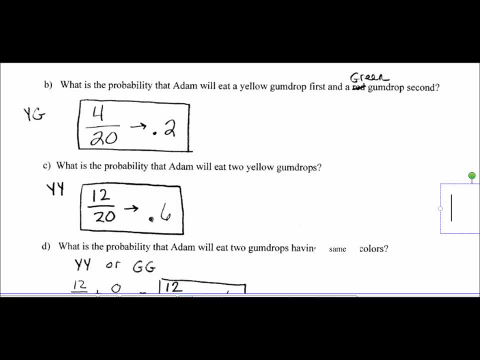 That's four out of twenty. What's the probability that Adam will eat two yellow gumdrops? Well, that's given by Y Y yellow, yellow. twelve out of twenty. What's the probability that Adam will eat two gumdrops of the same color? 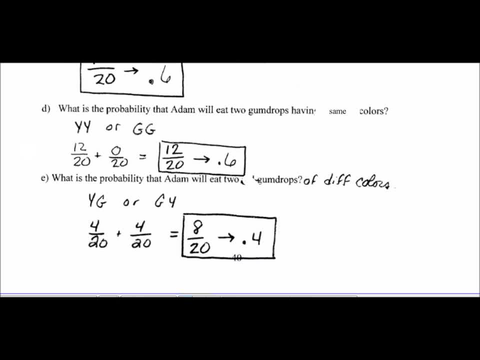 That happens with yellow, yellow or green green Twelve out of twenty, or which is plus zero out of twenty, There's a twelve out of twenty chance. Finally, what's the probability that Adam will eat two gumdrops of different color? 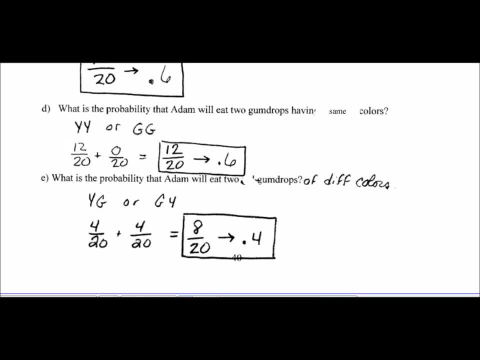 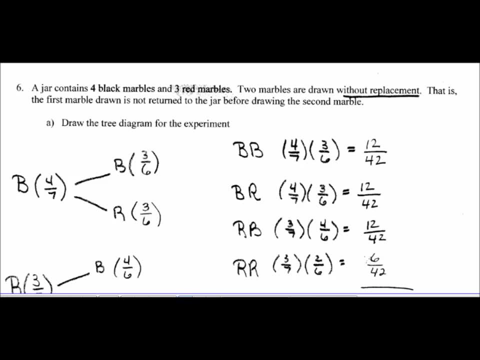 Well, that happens when we have Y G yellow green or G Y green yellow. That's an eight out of twenty chance. The next page: we have Jack, we have a jar and there are four black marbles, three red, 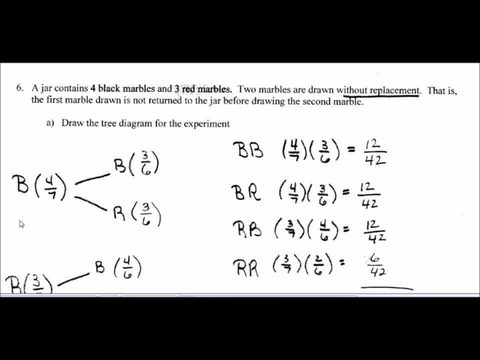 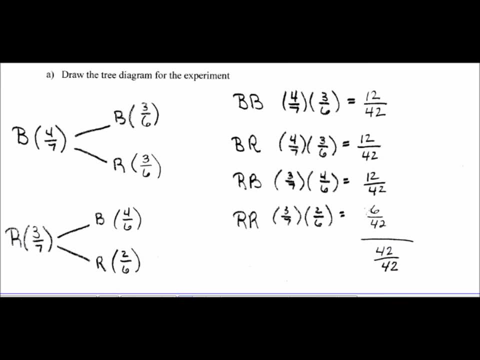 Two marbles are drawn out without replacement, And so the tree diagram illustrated here shows the probabilities associated with all the possible events: Black, black, black, red, red, black and red red. We use those probabilities listed over in our sample space on the right hand side to: 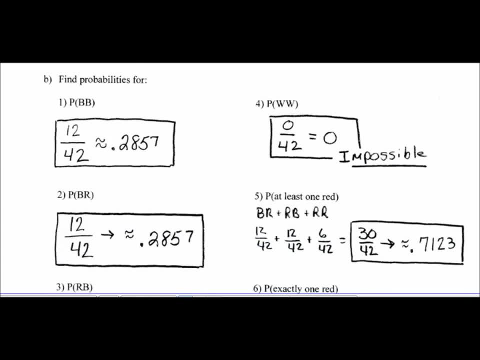 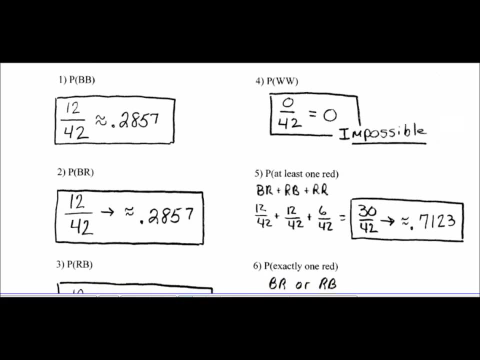 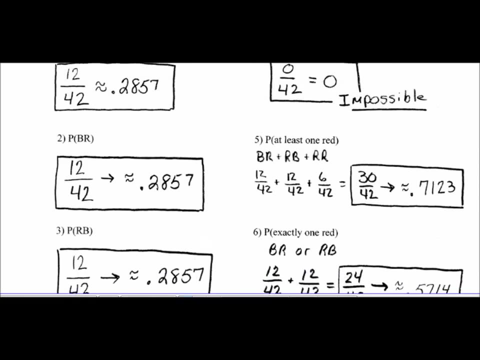 answer the questions that follow. The probability for black and black is twelve out of forty-two. Probability for black then red: twelve out of forty-two. Probability for red then black. also twelve out of forty-two. Probability of white then white. well, hey, there are no white marbles, so that's impossible. 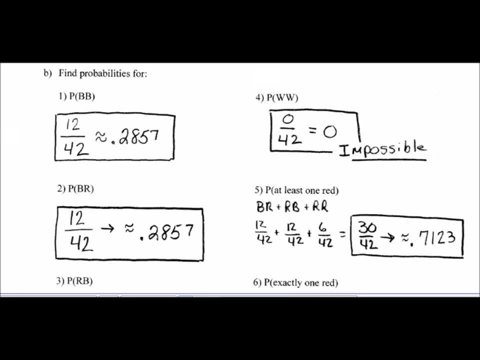 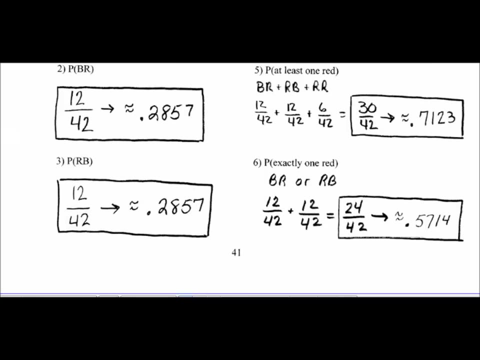 Zero probability. Probability of at least one red. at least one means one or more. That happened with blue, red, red blue and red red. I'll add those three probabilities together, thirty out of forty-two. And the probability of exactly one red happened with B, R or R B. twenty-four out of forty-two. 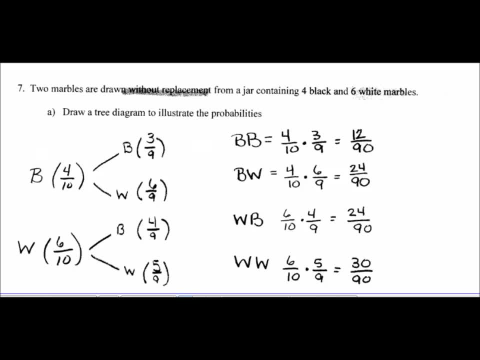 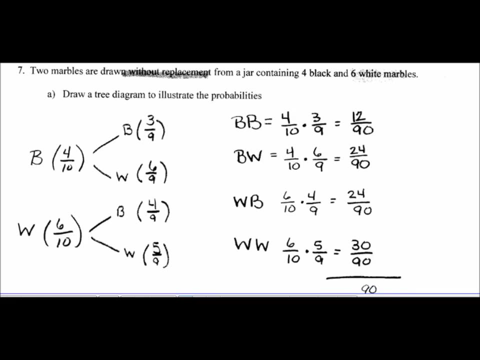 Finally, we have two marbles drawn, without replacement, from a jar. This time we have black and white marbles. We have a tree diagram that shows us the related probabilities, and off to the right hand side we have our sample space. We use those to answer the questions that follow.